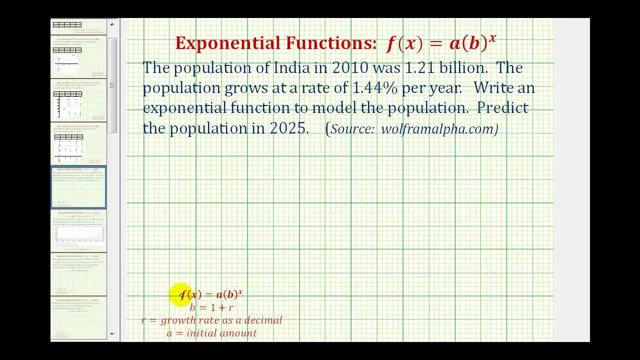 To model this population growth. we're going to use the exponential function in this form here: f of x equals a times b raised to the power of x, where the base b is equal to one plus r, where r is the growth rate expressed as a decimal. 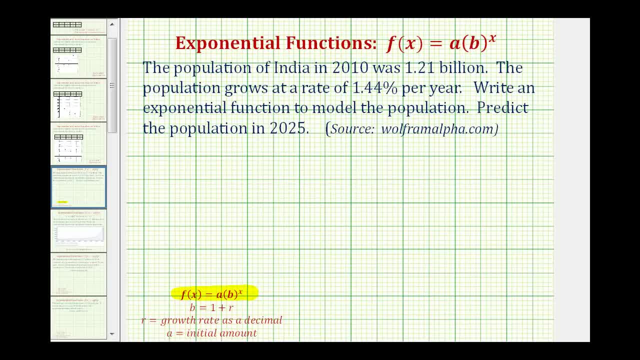 a is equal to the initial amount, or, in this case, the initial population, and because our function will be in terms of time, the exponent x would be the number of years after the base year. I do want to point out that, for this problem, 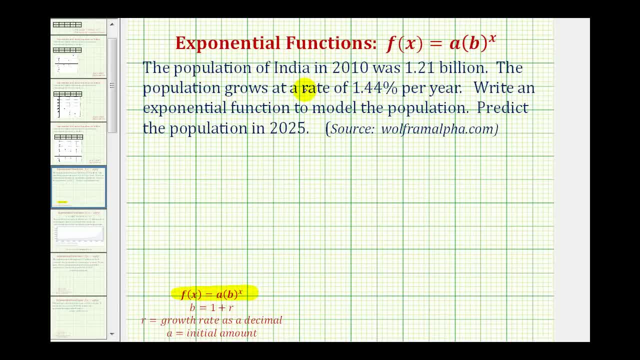 we're not told. this growth rate is a continuous growth rate and that's why we're using this exponential function rather than the exponential function with base e that we use for continuous growth. Just to illustrate that this population is exponential, here's the graph of the population of India over time. 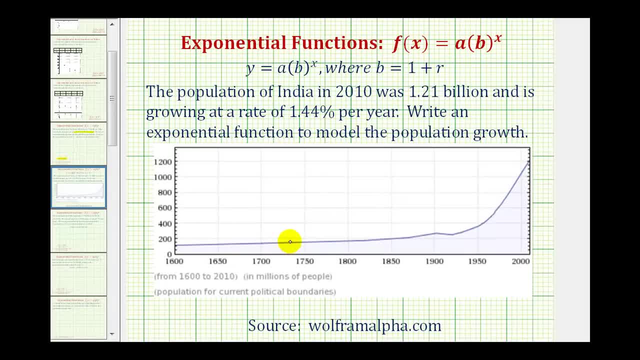 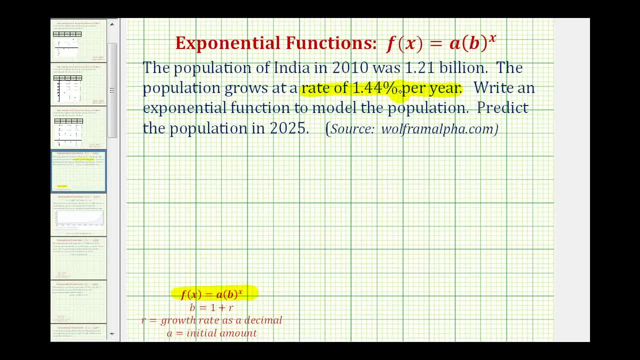 And you can see from the graph, an exponential function is an excellent model to model this population growth. So, going back to our problem, because our function represents the population of India, we're going to write a function, p in terms of t, where t is going to be the number of years. 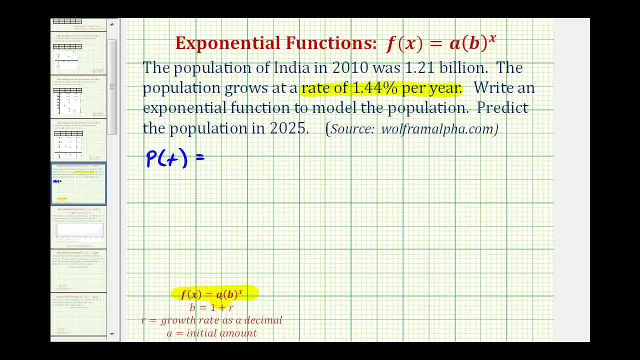 after the year 2010.. Again, a is the initial amount or, in this case, the initial population. so that'll be 1.21 billion plus the annual growth rate expressed as a decimal. So right now we have r equals 1.44 percent. 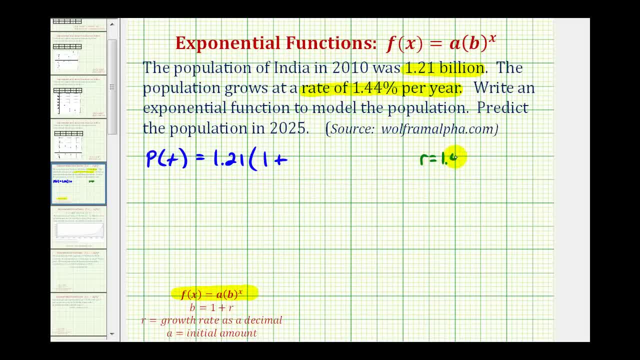 As a decimal, that would be 0.0144.. So we have 1 plus 0.0144 raised to the power of t. Let's go ahead and simplify this. We have p of t equals 1.244.. So we have 1 plus 0.0144 raised to the power of t. 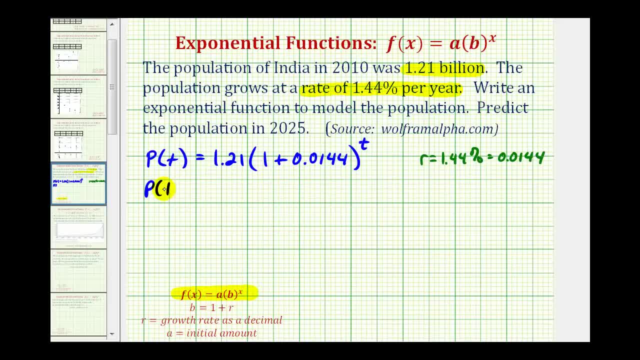 Let's go ahead and simplify this. We have p of t equals 1.0144 raised to the power of t. So we have 1.21 times 1.0144 raised to the power of t. So p of t will be the population. 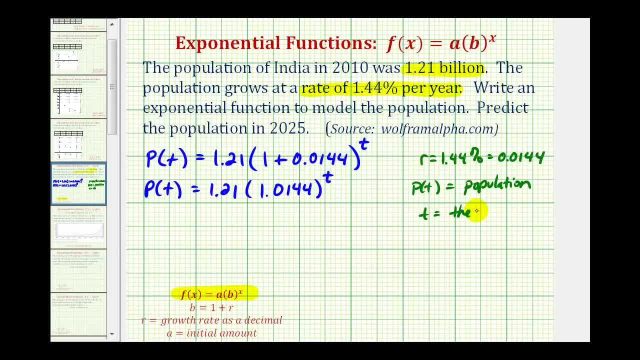 and t will be the number of years after our base year of 2010.. So here's the function that we can use to model the population of India And to predict the population in the year 2025, we need to determine what value of t to use.